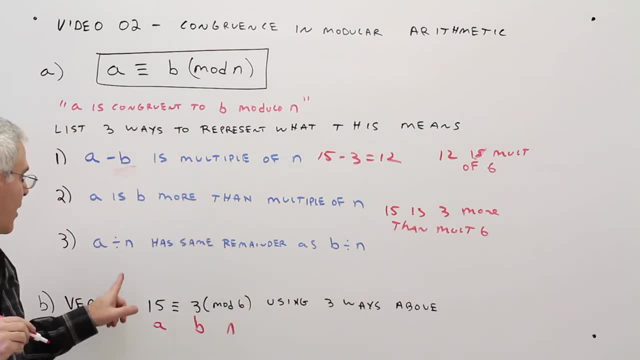 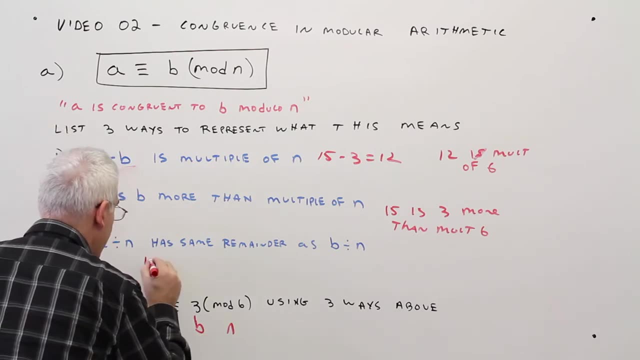 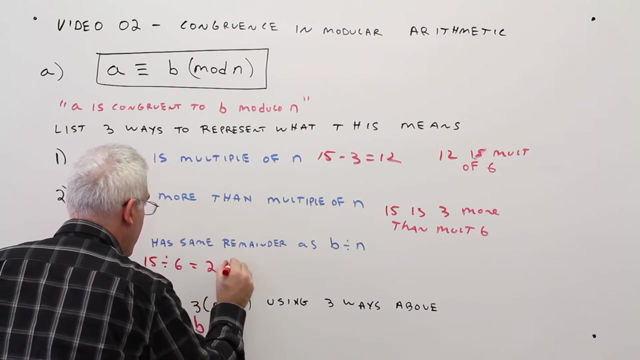 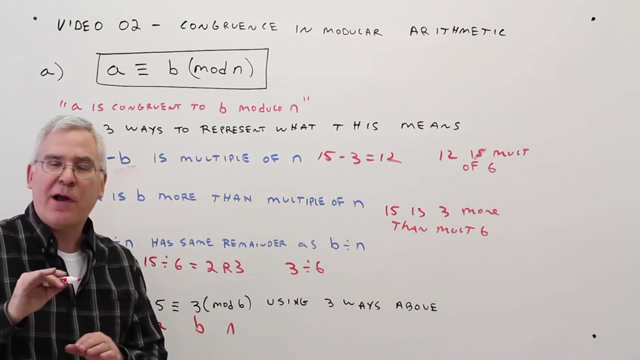 is a multiple of 6, and 12 plus 3 is 15.. Over here, A divided by N has the same remainder as B divided by N. All right, so 15. Divided by 6 equals 2 remainder: 3.. Now I'm going to go. 3 divided by 6.. Now, just to make sure that. 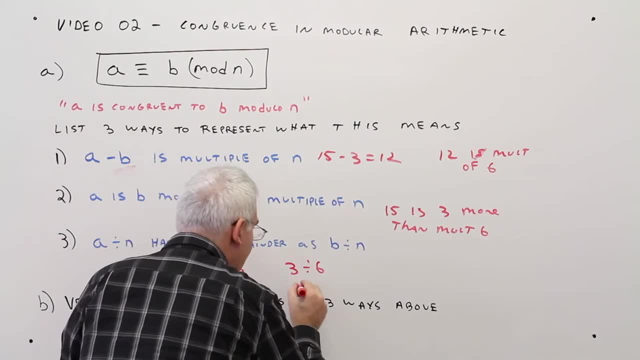 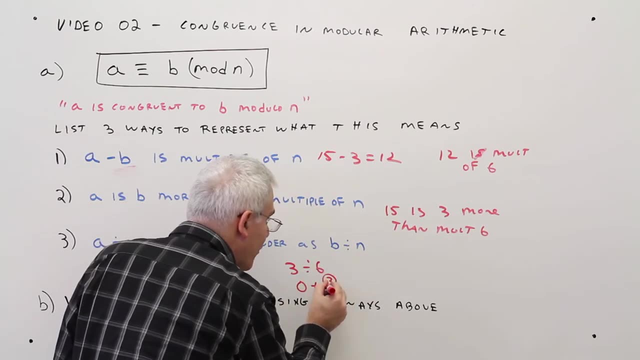 we're extra clear: 3 divided by 6 is the same as 0 plus 3 over 6.. And then, of course, whatever is in that numerator is the remainder. So 3 divided by 6 equals 0 remainder. 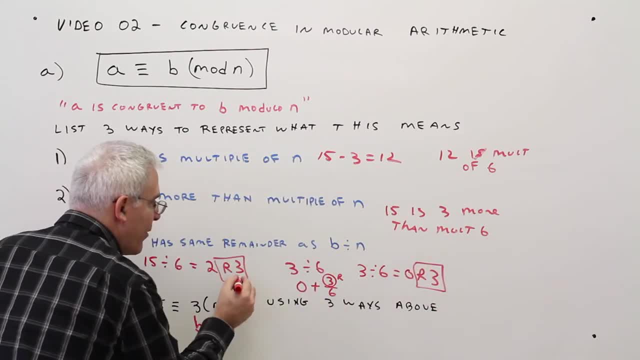 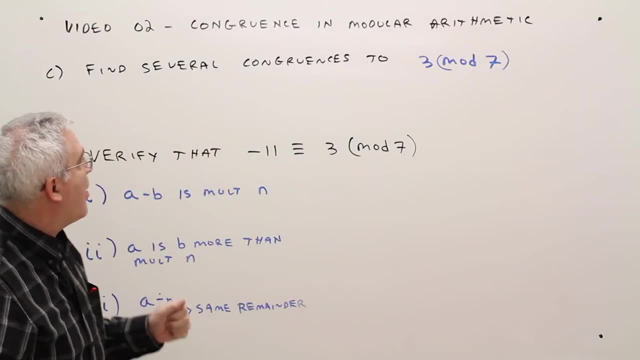 Remainder 3.. So I've got a remainder 3 there and a remainder 3 there, and those remainders are the same. Okay, I'm going to do problem C now. Find several congruences to 3, mod 7.. All right, 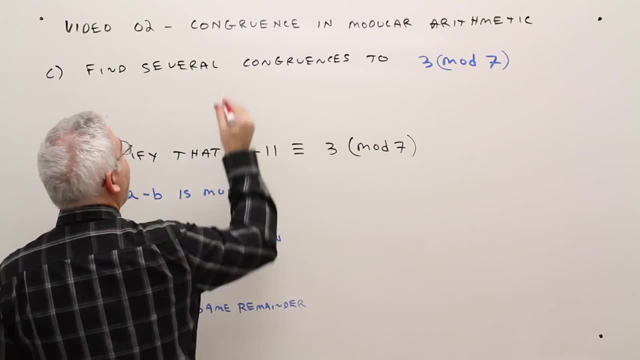 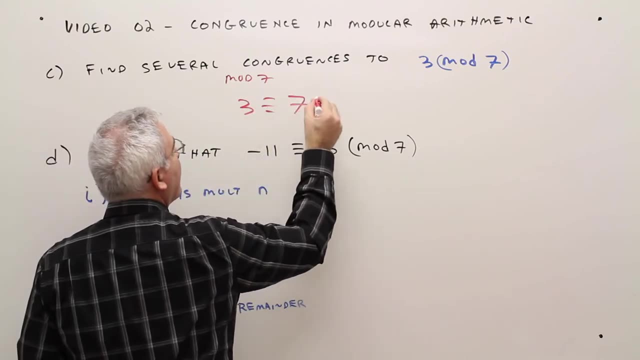 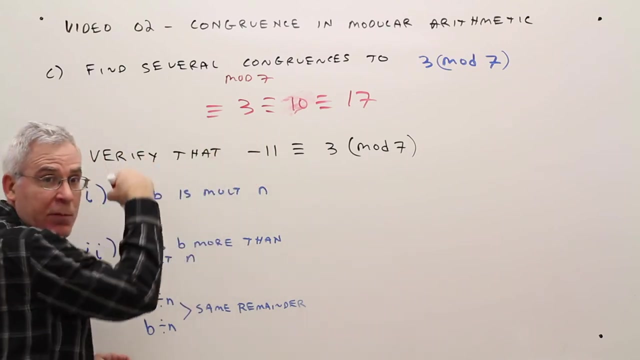 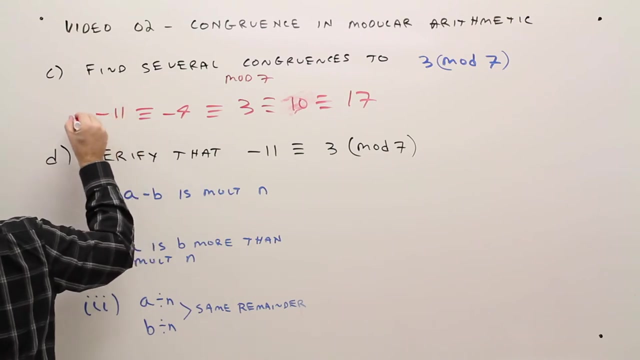 so I just want to emphasize that we're in mod 7.. So 3, we can just keep adding 7.. 10, adding 7. 17.. Subtracting 7, negative 4.. Subtracting 7, negative 11.. And this pattern goes on. 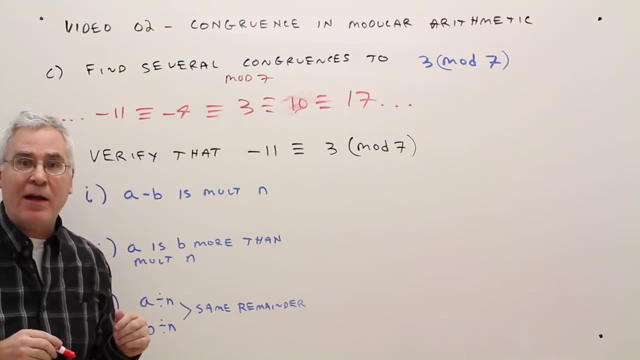 infinitely. All right, and again I'm stressing, I'm in mod 7.. Now what I want to do is verify that negative 11 is congruent to 3 in mod 7 by the three methods outlined previously. All right, so let's just do some labeling. This is the a value, the b value and the n value, So a. 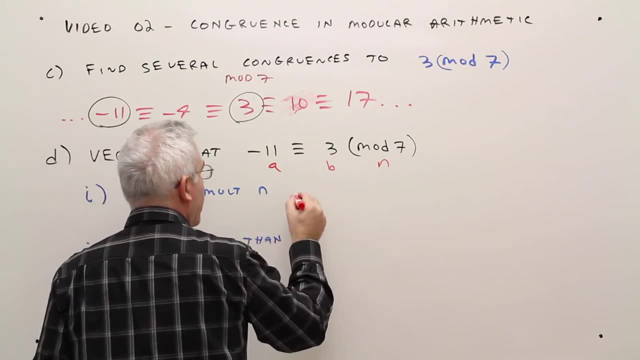 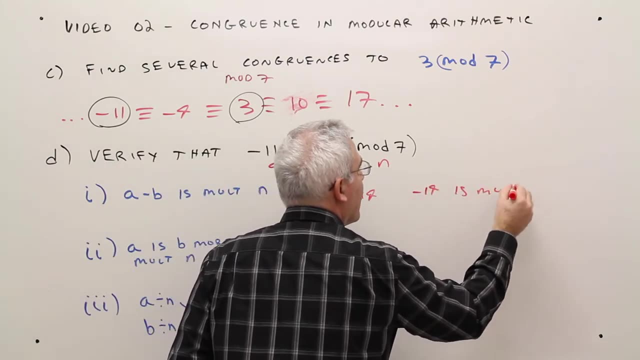 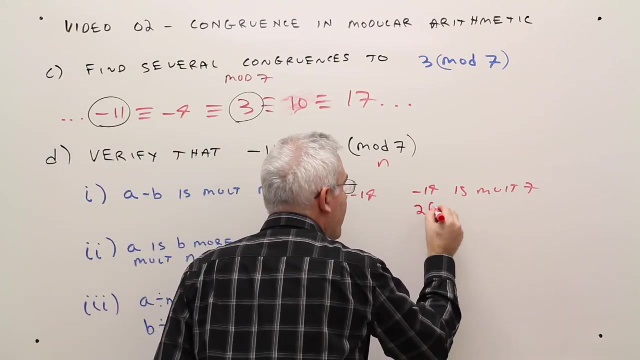 minus b, let's see if it's a multiple of n. So negative 11 minus 3 is negative 14.. And negative 14 is a multiple of 7.. Negative numbers are multiples. I can prove it by saying 2, or negative. 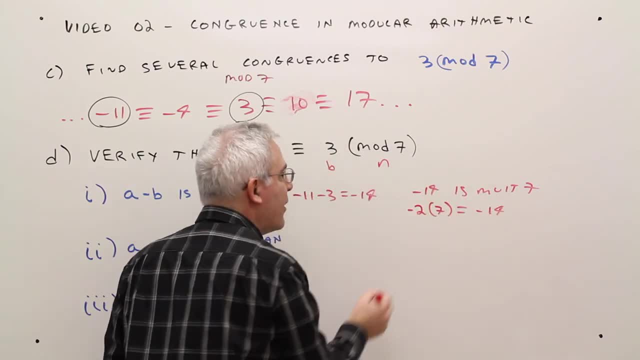 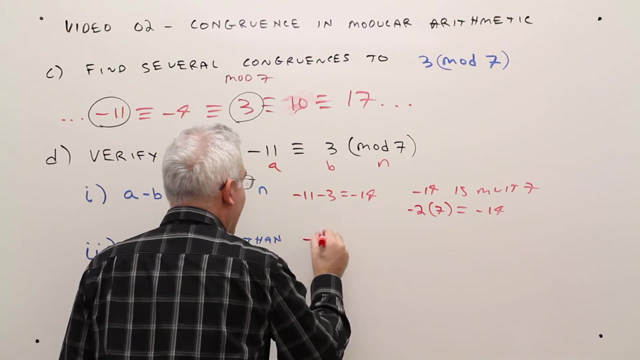 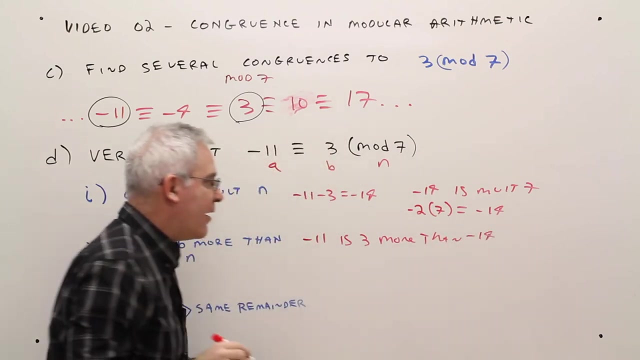 2 times 7.. So negative 14 is a multiple A is b more than a multiple of 7.. All right, so negative 11 is 3 more than negative 14.. And negative 14,, of course, is a multiple of 7.. And then this last one I want to.